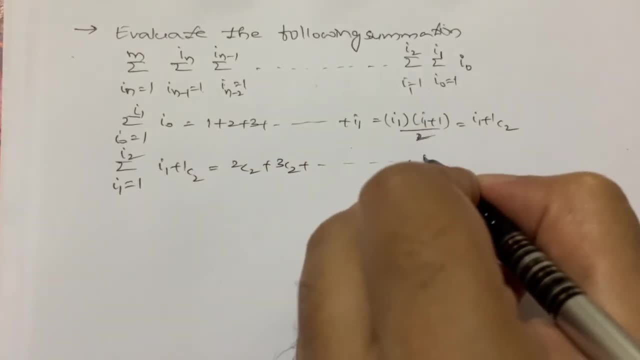 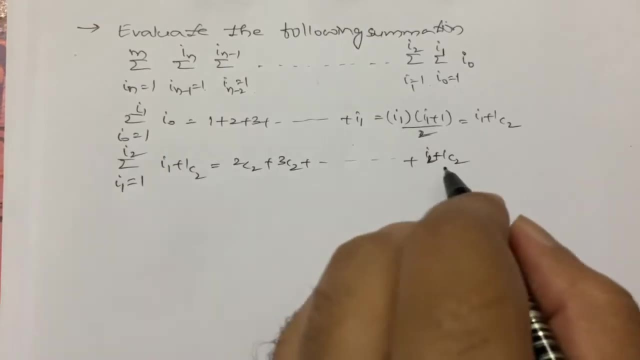 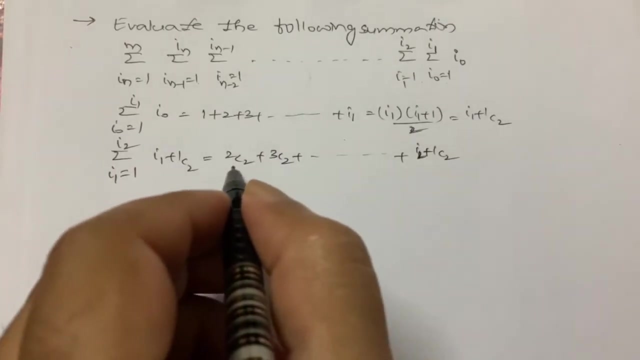 plus 3 C 2, so on to I 2 plus 1 C 2.. So if I want to find this, so this summation we want, so for that what we can do is we will use this, So this we can write as 2 C 2 can. 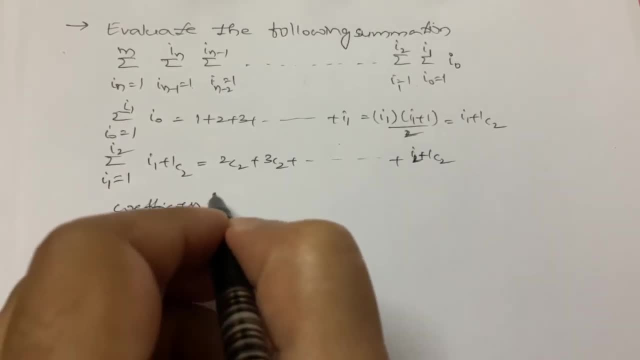 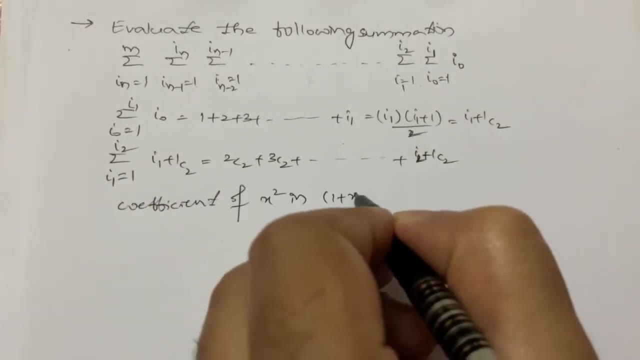 be written as coefficient of, so here all suffixes are 2, so coefficient of x square n, So 1 plus x whole square. if I write 1 plus x whole square, 2, C, 2 x square, I will get here: 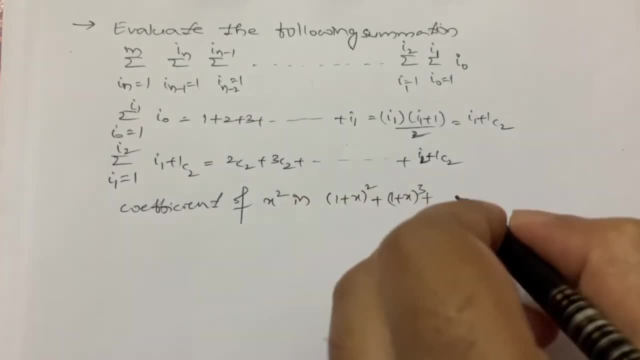 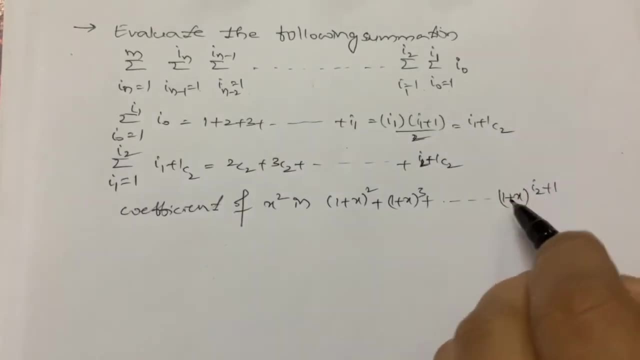 1 plus x, whole cube, 3, C, 2, x square, so on: 1 plus x, whole power, I, 2 plus 1.. So I 2 plus 1, C 2 is the coefficient of x square here. So if I want to simplify this, so this is: 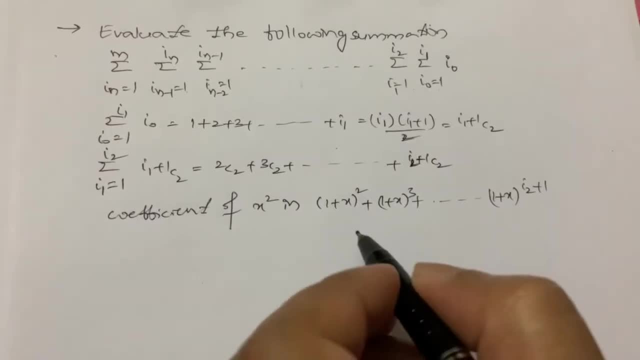 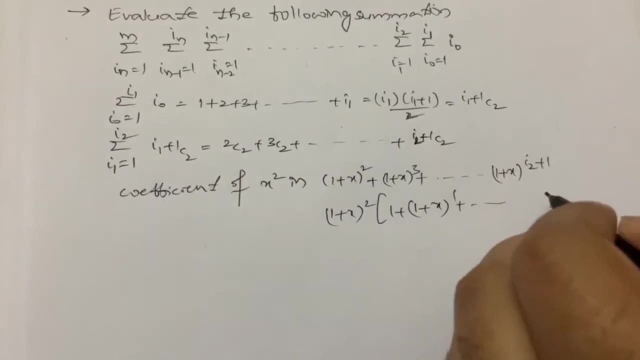 g, p, right clearly. So the common ratio is 1 plus x. So 1 plus x whole square into 1 plus 1 plus x power 1, so on 1 plus x, power I, 2 minus 1.. So this is 1 plus x, square into. 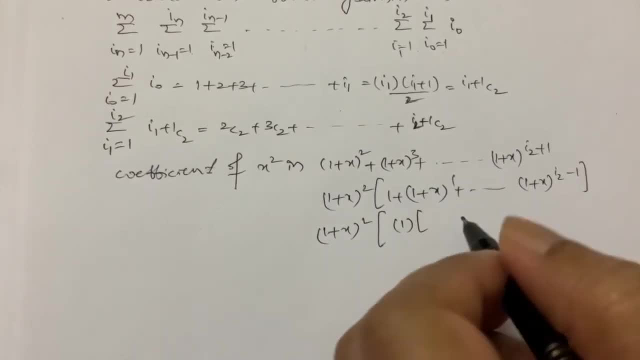 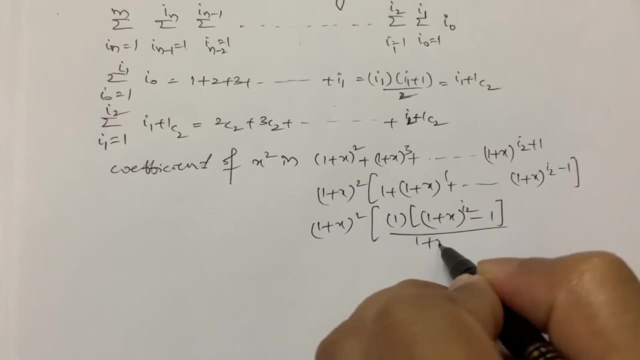 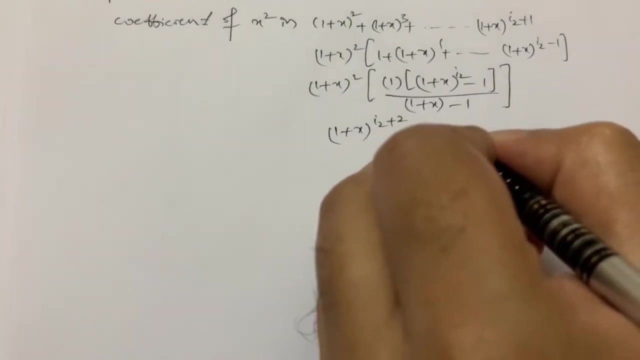 so a into a is 1 r power n. So 1 plus x power I 2, because I 2 terms are there minus 1 by 1 plus x minus 1.. So this is 1 plus x power I 2 plus 2 minus 1 plus x, whole square by: 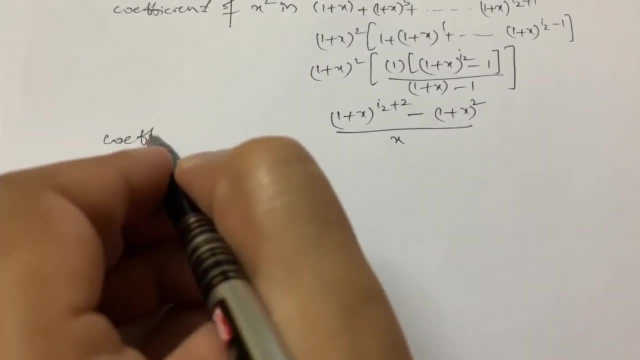 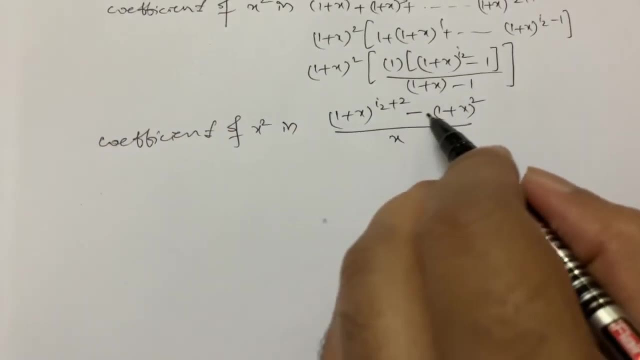 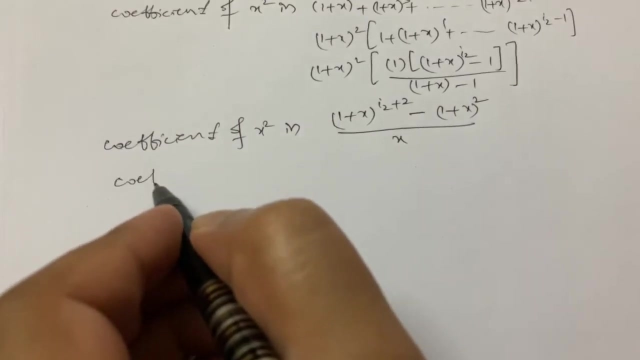 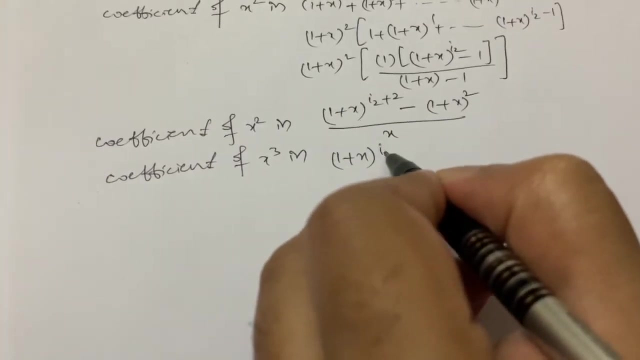 x. So we want coefficient of x square, right, but here denominator x is there. So it means, if I want x square here, I have to find x cube coefficient here. So this: to avoid x in denominator, coefficient of x cube in 1 plus x, whole power I: 2 plus 2 minus 1 plus. 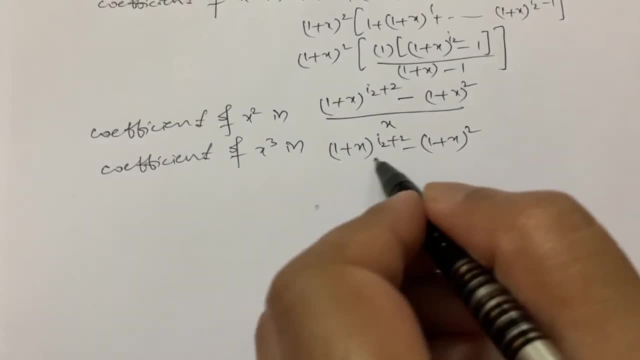 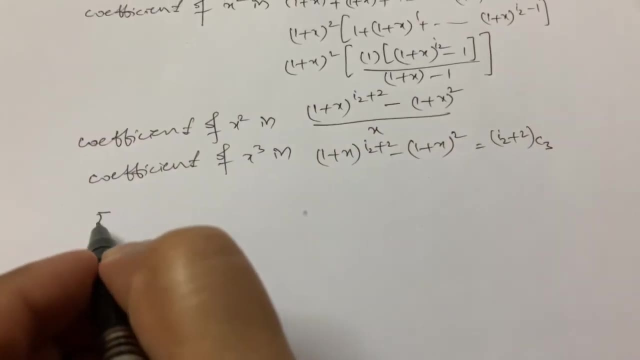 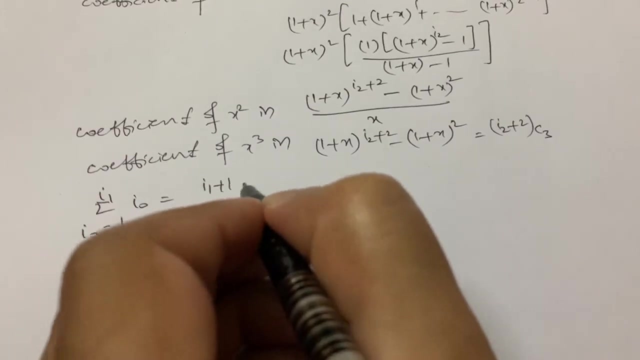 x whole square. So here cube coefficient will not be present, So here only we will get So which is I 2 plus 2 C 3.. Let us look at the first summation sigma: I naught equal to 1 to I 1. I naught is equal to I 1 plus 1 C 2.. And the second: 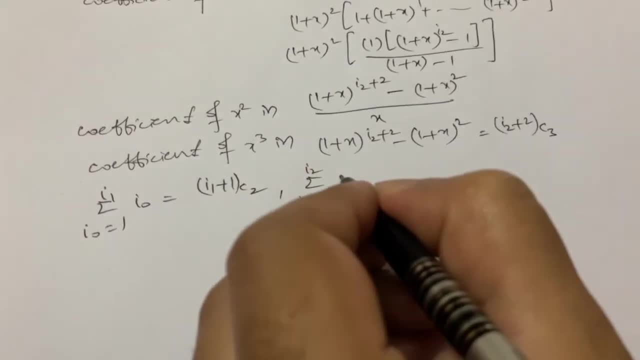 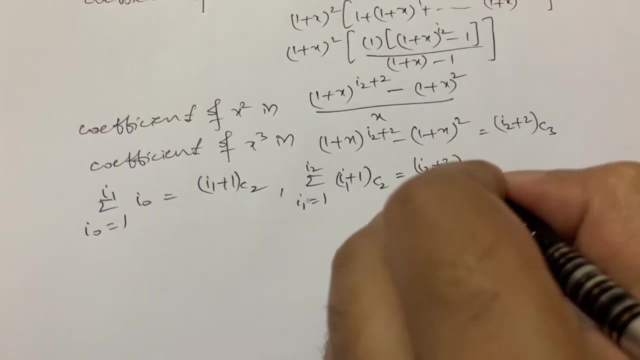 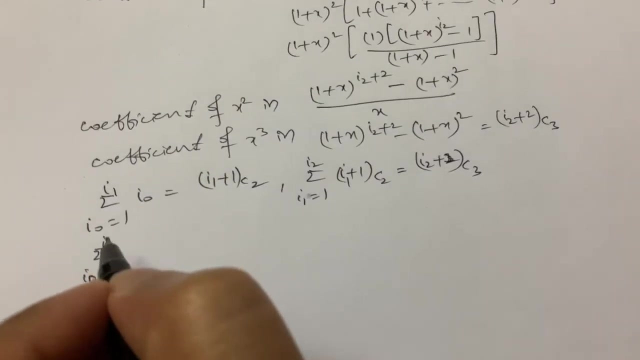 summation: sigma I 1 is equal to 1 to I 2. I 1 plus 1 C 2 is equal to I 2 plus 3, C 3, I 2 plus 2, C 3.. So first we will, and in the first summation, so I naught, I can write as I naught: C 1,. 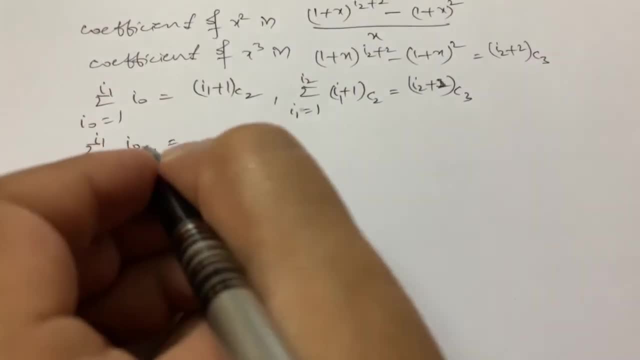 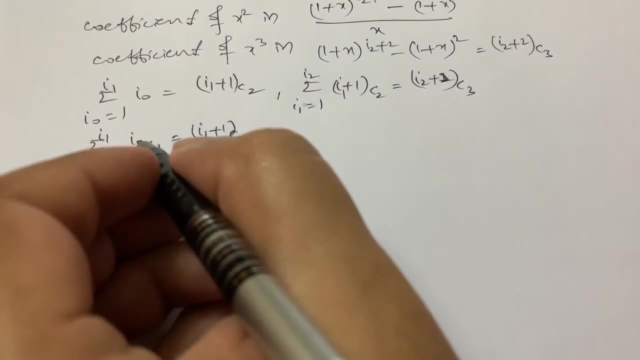 I naught we can write as I naught: C 1.. So if we are writing I naught C 1 summation, we are getting I 1 plus 1 C 2. So we are increasing. I naught I mean the highest power. 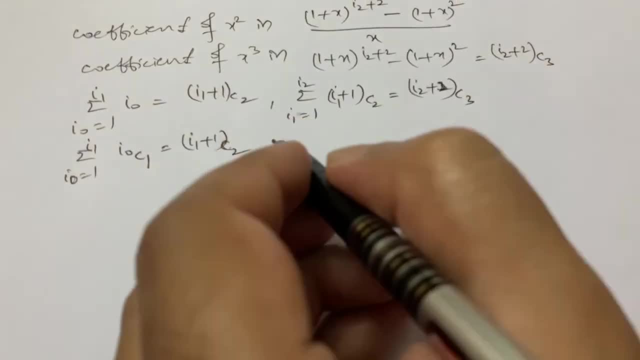 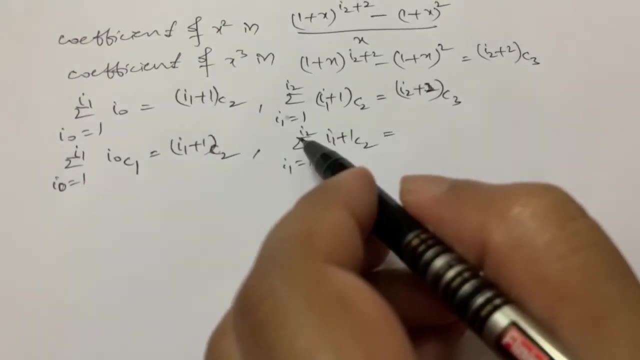 plus 1 C, 1 plus 1.. So if you see the second summation, I 1 is equal to 1, 2, i 2. i 1 plus 1 c, 2.. So now the highest term is i 2.. So we have to increase. 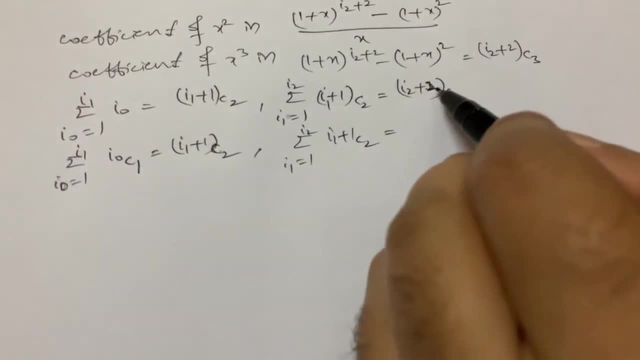 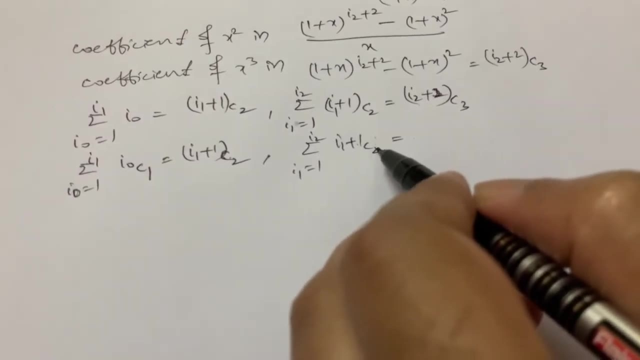 by 1.. So if I increase by 1 i 2 plus 2, because i 2 plus 1 plus 1, we have been increasing, So here also 1, we are adding, So c 2 plus 1.. So this is i 2 plus 2, c, 3. So similarly, 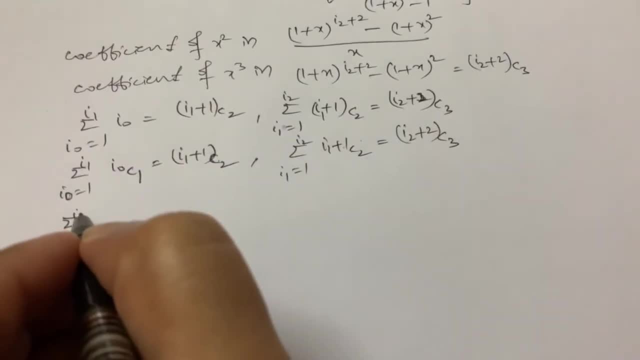 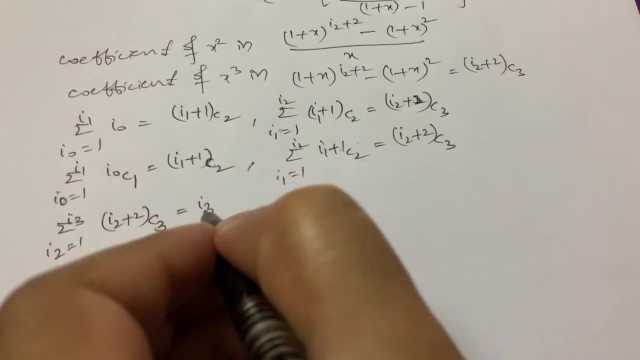 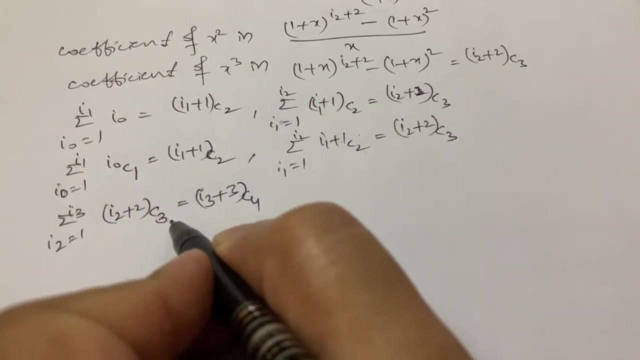 the third summation will be: i 2 is equal to 1, 2, i 3. i 2 plus 2, c 3 will be i 3 plus 3, c 4, because we have to increase the highest by 1, and then here we have to increase by: 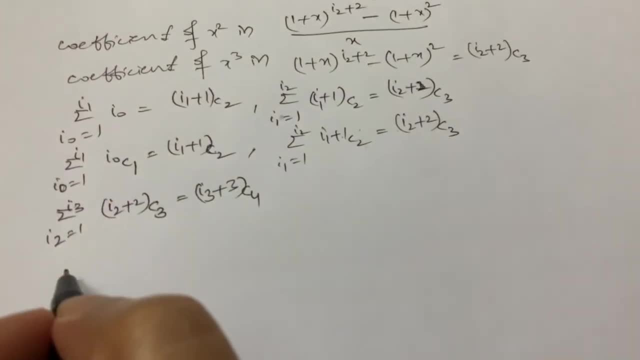 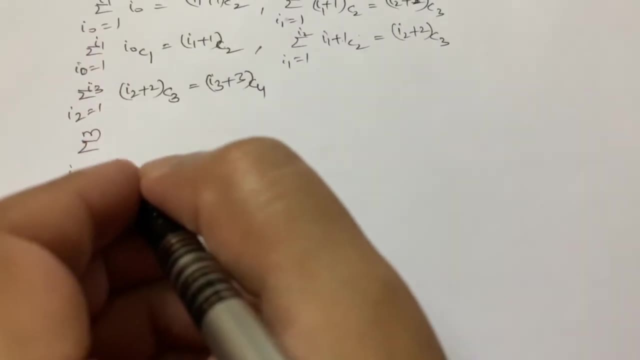 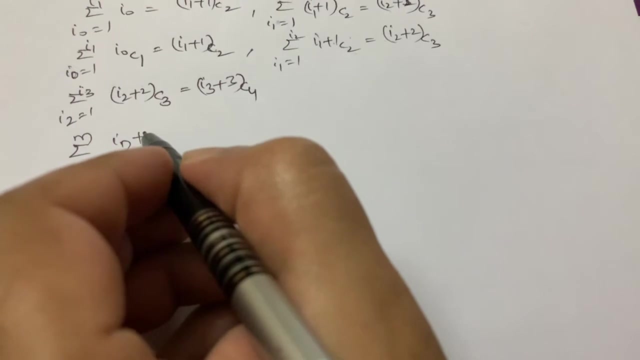 1. So similarly, if I do all summations, the final summation is sigma. i n is equal to 1, 2 m. So for the final summation we will get So 2.. So what we will get here: I n plus n, c, n plus 1, that is what we will get, So the highest. 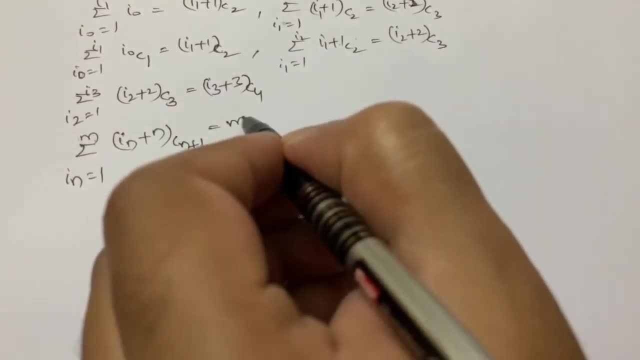 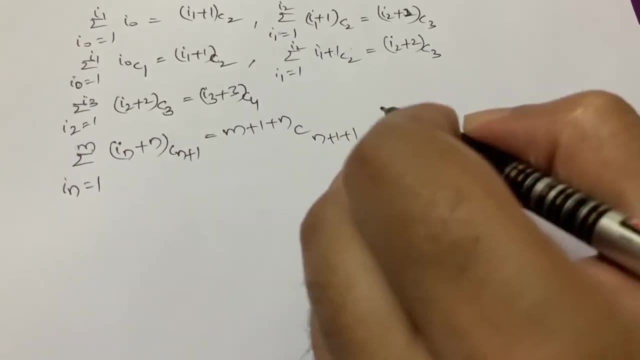 power here. highest term here is m, So this m plus 1 plus n c. we have to upgrade this by 1 n plus 1 plus 1.. So this is m plus n plus 1 c, n plus 2.. So the final summation.